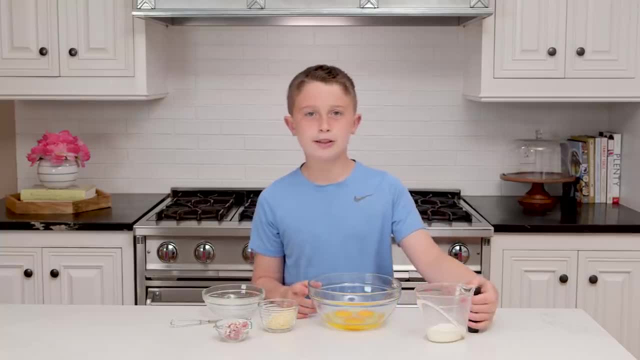 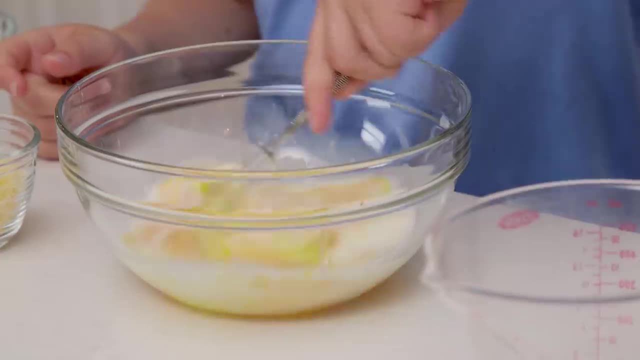 20 seconds. Okay, next I'm gonna pour my milk in and then give it a big whisk, And I use this milk because it keeps it really fluffy: Whisk, whisk, whisk. Okay, so my eggs are looking pretty good. 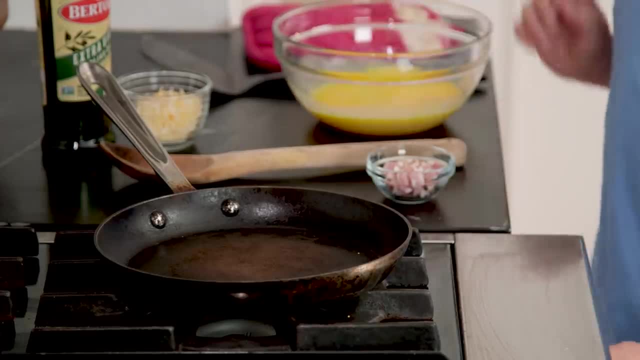 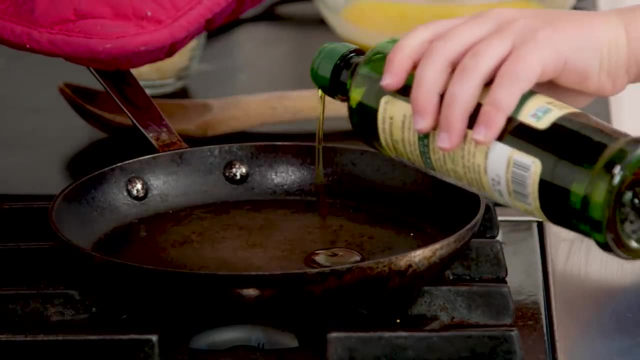 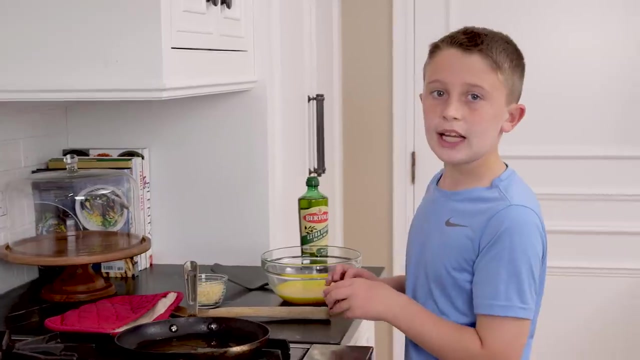 Now it's time to move over to the stove, So I am going to heat up my pan. Let's put some olive oil on there so that nothing sticks. So you want to give your pan a second to heat up And then, once you think it is hot enough, you can go ahead and add your pancetta. 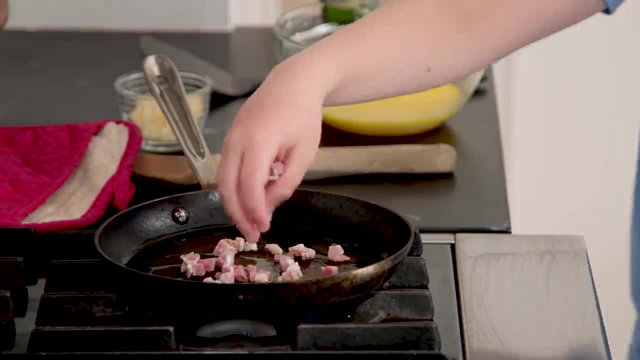 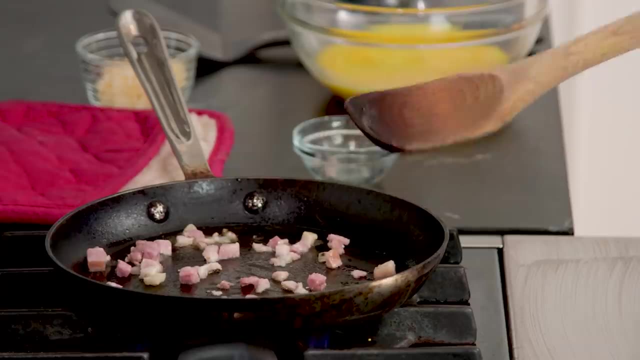 Pancetta is a little bit like bacon, but not quite bacon. It's really good and it goes really well in omelets. I find You can hear that nice sizzle. It sounds really cool. I'm going to give it a chance to cook up. 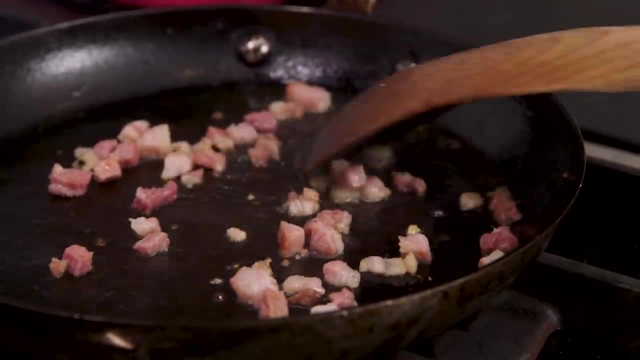 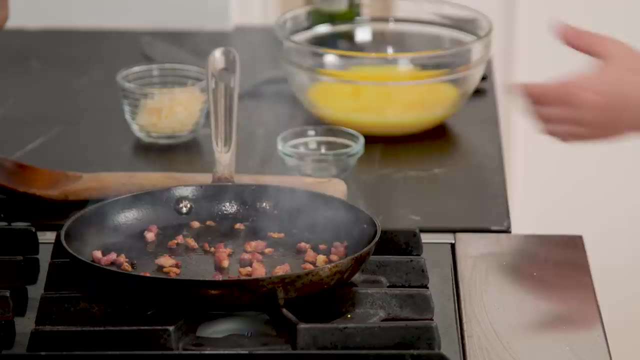 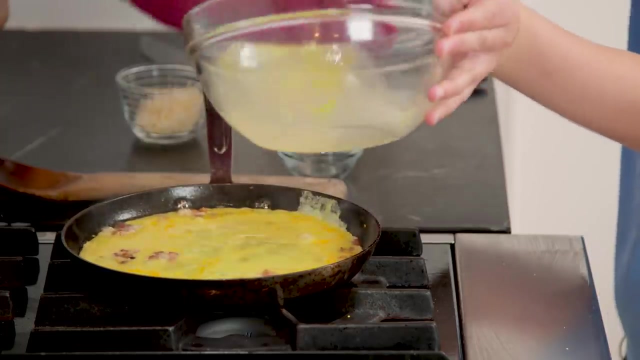 Sometimes it actually starts to pop like popcorn, which I think is cool. I think my pancetta is looking good, So I'm going to turn down the heat and pour in my eggs that I just whisked. Okay, my heat is turned down and I'm going to start scraping parts from the egg. 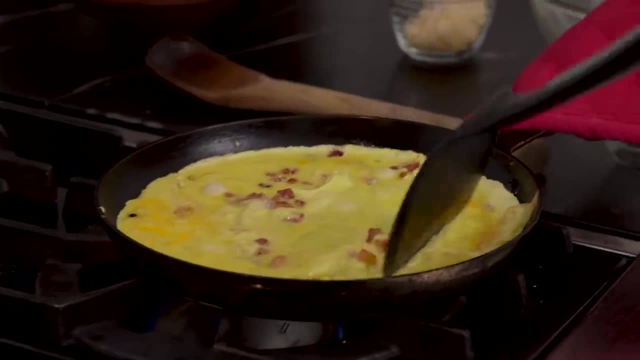 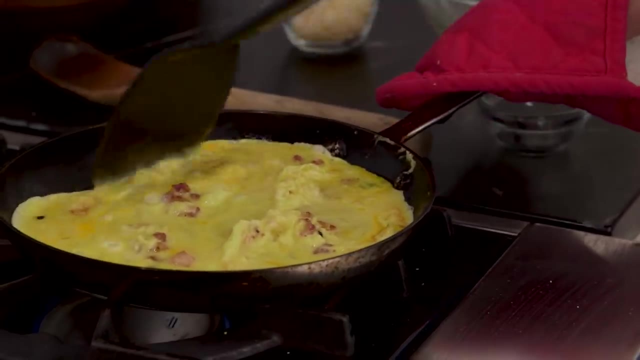 From the outside to the middle and then filling that outside part back in. This is one of the reasons why I turn my heat down, Because it might not have enough of this liquid to fill in all the gaps if my heat is too far up. 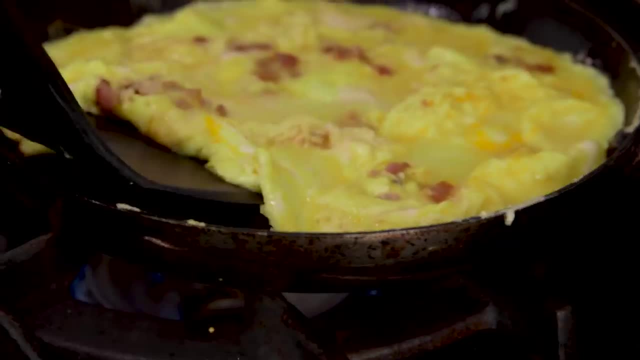 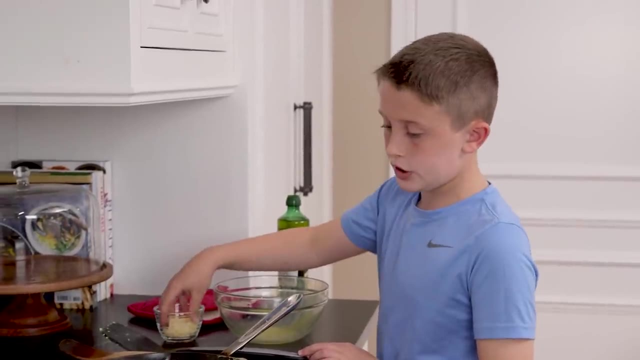 Once it cooks a little bit longer, you can kind of check it. It's about to be ready, but not quite yet. That's looking pretty good. I think I'm ready to put my cheese on now. I like a lot. You can do a little. You can do a lot. You can do right in between. 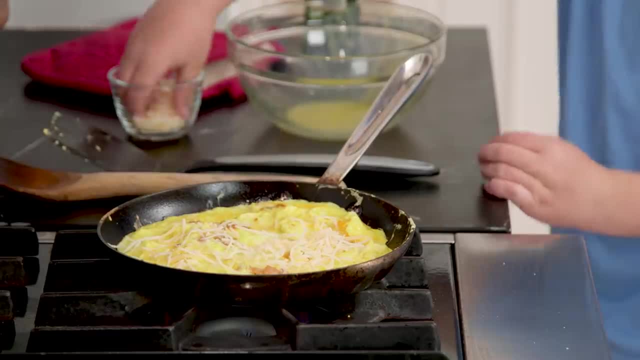 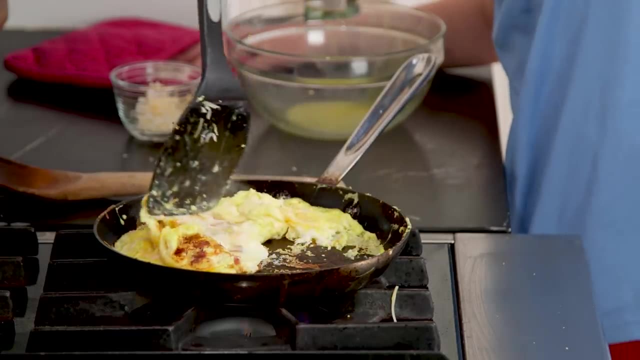 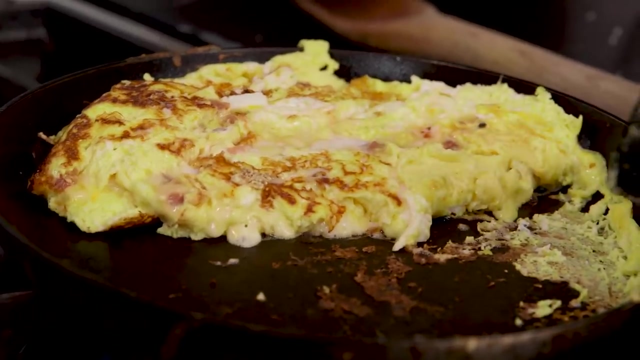 This part could get a little messy, But that's fine, because in the end an omelet is an omelet and it doesn't need to look perfect. So I'm going to flip this now. Fold it over And you can see that the cheese coming out of the sides. 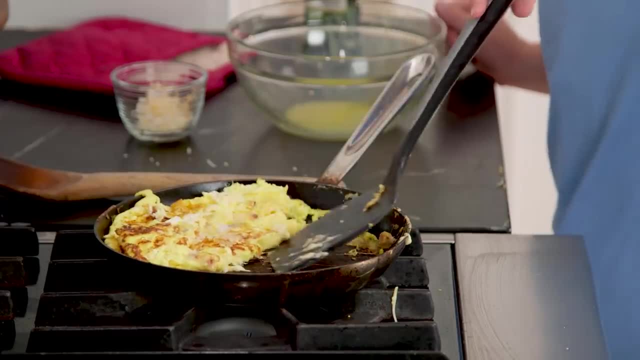 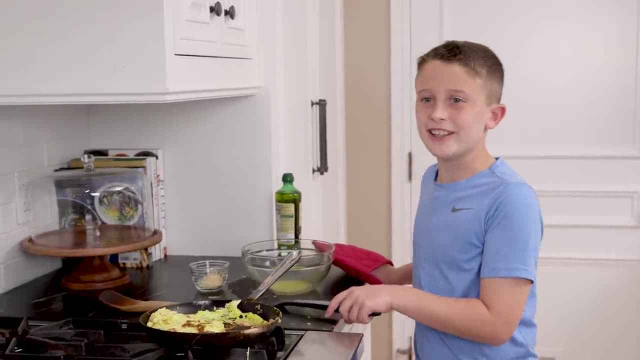 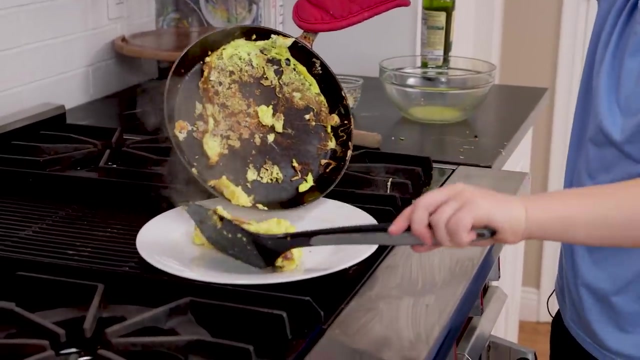 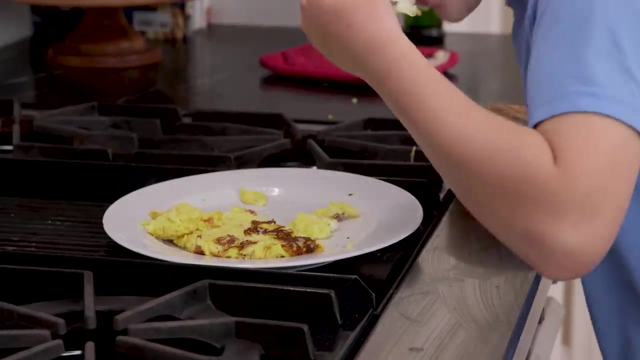 As the final step, cook it a teeny bit on the other side. I think this is looking pretty good. Let's get this plated up and dig in. I made this with a little salt and then dig in. This is pretty darn good. 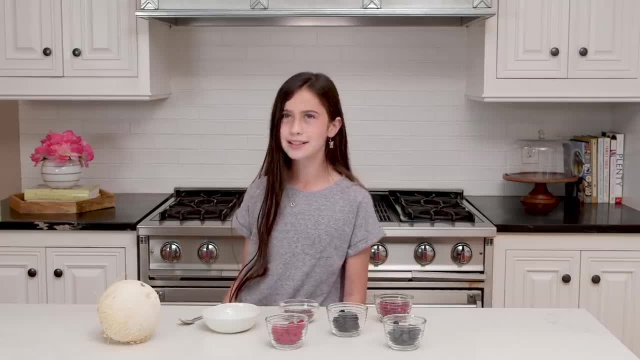 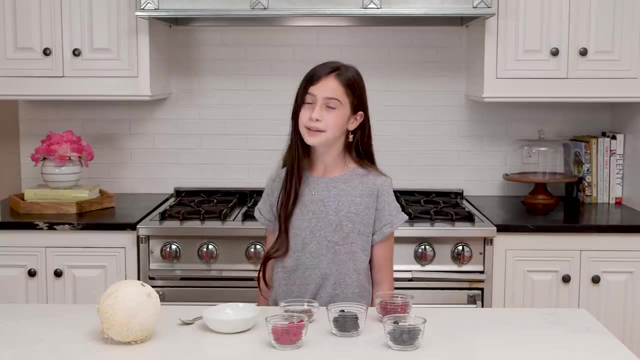 Finally, we are going to be making nature's cereal. I know we said no cereal, but I'm going to make an exception- So you've probably seen this before- because it's kind of viral right now, But we're going to make it my way. 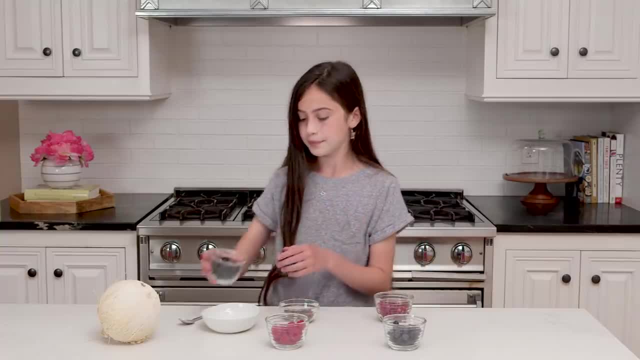 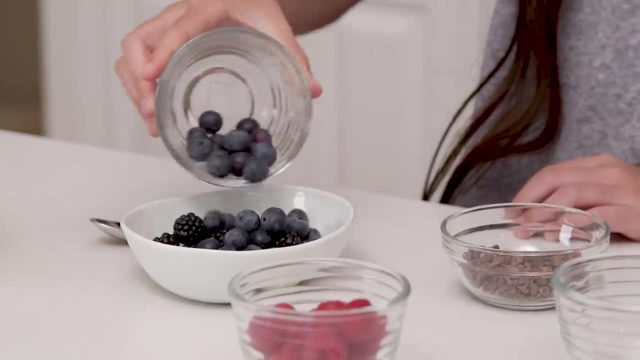 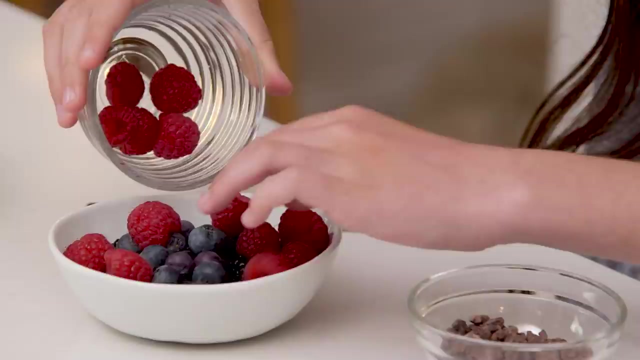 First I'm going to add my blackberries, Next I'm going to add my blueberries. You can really have any berries, but I chose these because it has a nice pop of color. Next I'm going to do my raspberries, And then I like to do the smaller things on top, so they kind of show. 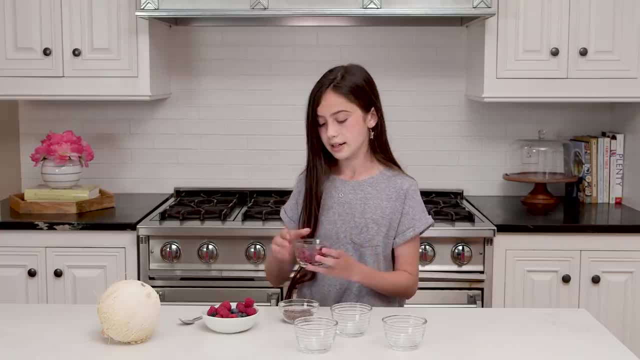 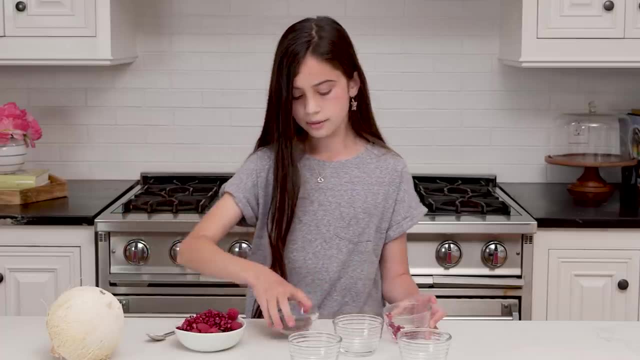 I'm going to be using pomegranate seeds And just going to sprinkle those guys on These. give you a nice crunch. Next, we are going to be adding some cacao nibs. This is my twist, because it can't be something for me if it doesn't have a little bit of chocolate. 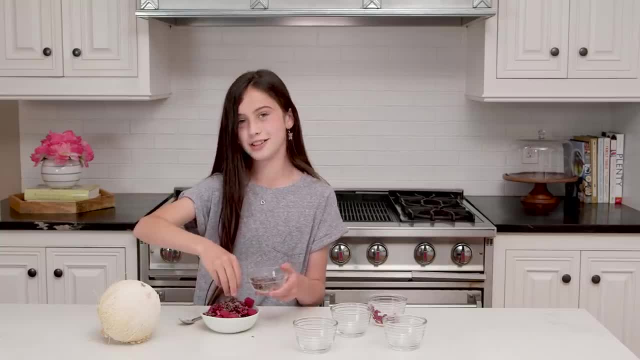 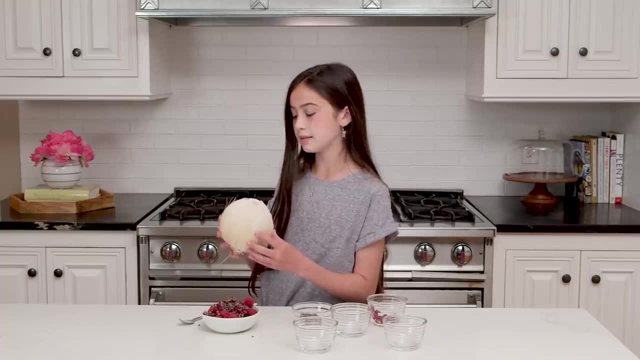 These are unsweetened, so they still count for nature's cereal. Okay, next we're going to do the coconut. You can always use the box coconut water, but I'm giving my mom splurge and get the coconut. I think I'm just going to have to shake it out. 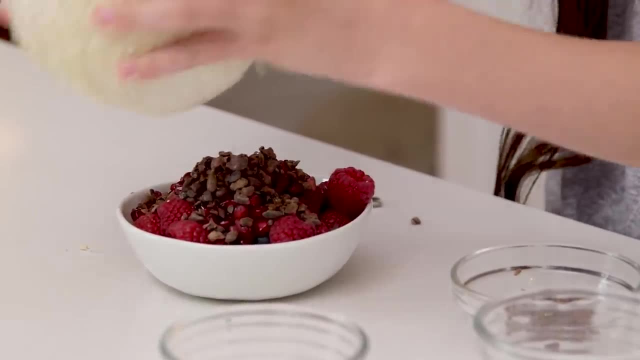 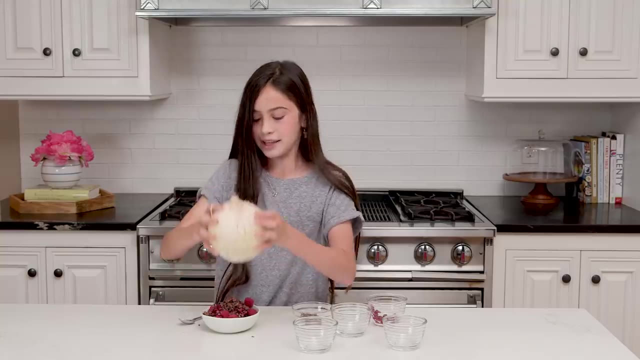 It could get messy, but it's going to be delicious. We learned in school about taking initiative, And taking initiative is cool. So after I'm done making this, I'm going to be cleaning this mess up. So I took the initiative to clean up my workspace and it looks pretty good. 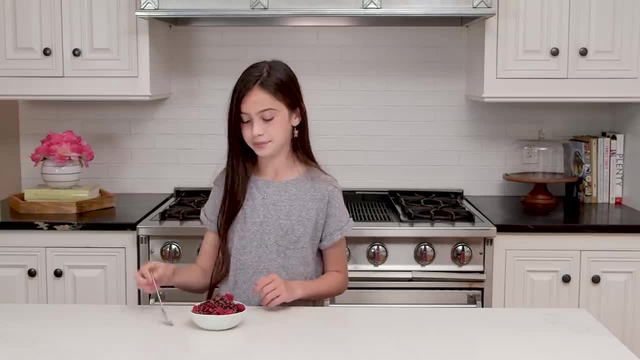 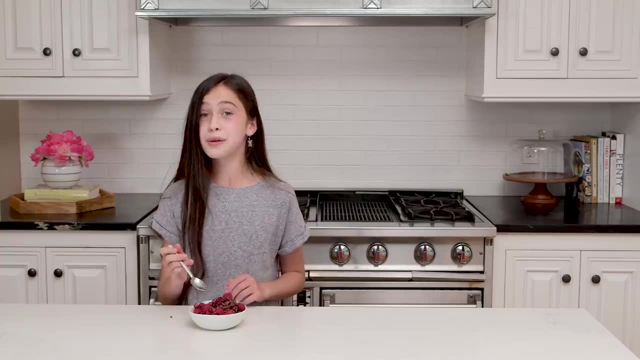 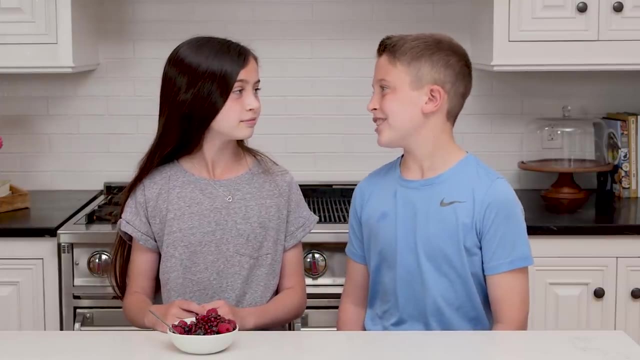 So now I'm going to try my nature's cereal, Going to get some of that nice fresh coconut water. That's pretty good. Who needs Captain Crunch when you got pomegranate seeds? I guess we should go wake mom up. Yeah, I guess we have to share some of this delicious stuff with her. 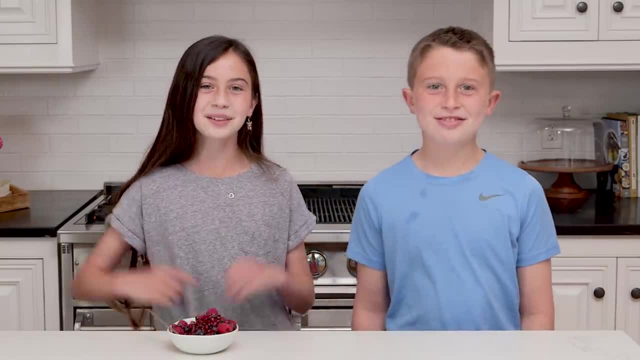 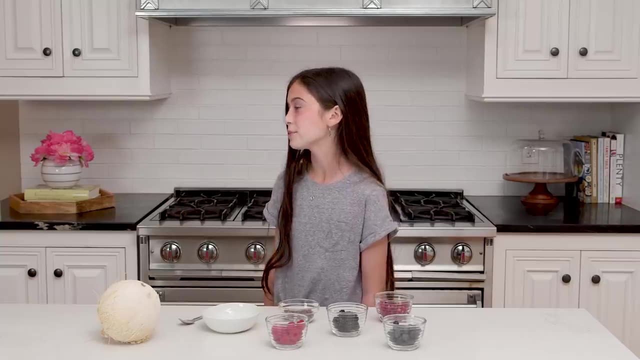 Yeah, Thanks for watching. Subscribe if you want to. Bye guys. Booyah, You going to save some for me? Probably not. No, I'm embarrassed by my brothers. Woo, Oh, I know, I know, I know.